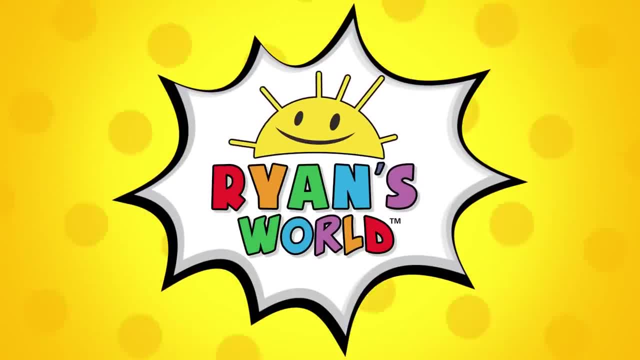 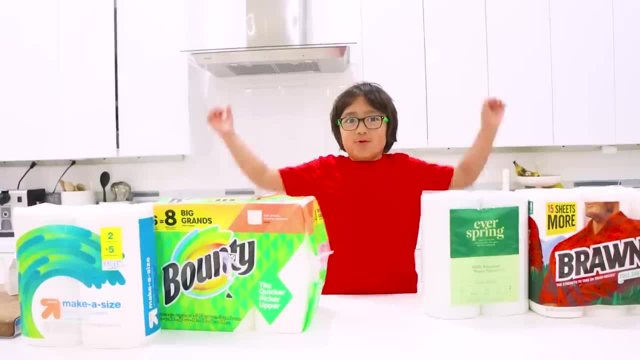 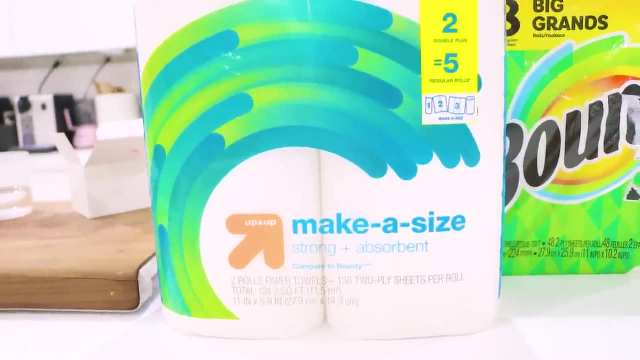 Welcome to Ryan's World. So we're going to test out all of these different brand paper towels and we're going to see which one's the most strong and most absorbent. We got this Target brand here that says make a size. It says strong and absorbent. 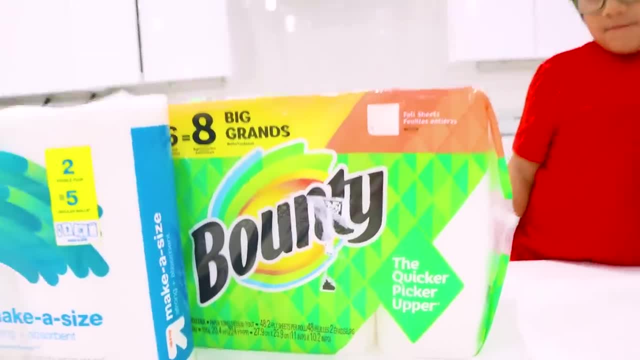 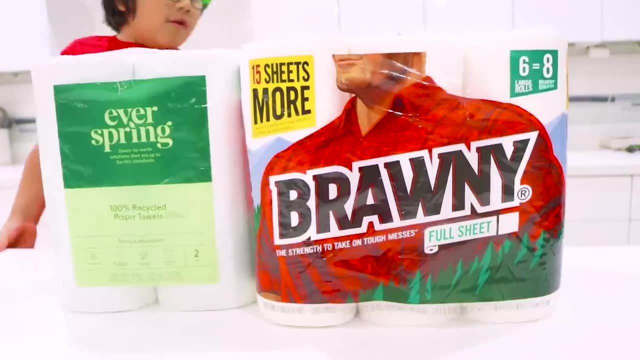 The Bounty brand. it also says the quicker picker-upper, so it's supposed to be really quick And this is the Recycle brand. and also it says strong and absorbent And a Bronte brand that also says the strength to take on tough greases. 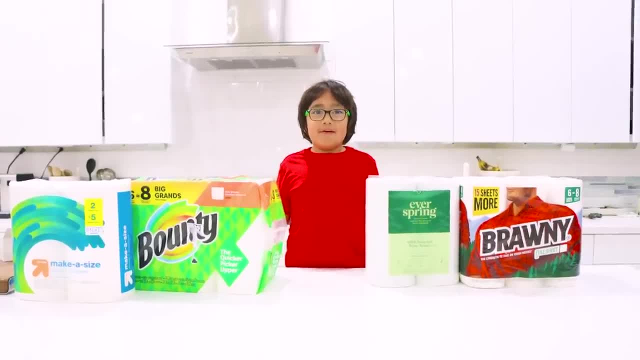 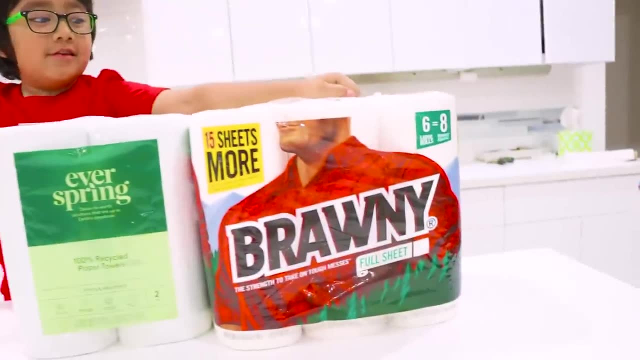 Out of all of these, which one, Ryan, do you think is the most strong and most absorbent? This one or this one? Oh really, The Bounty or the Bronte? All right, let's test it out, Yeah. 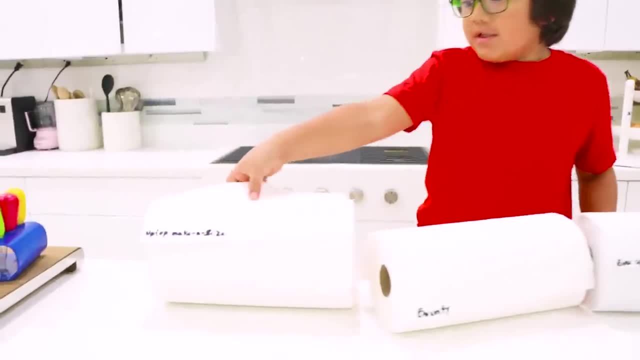 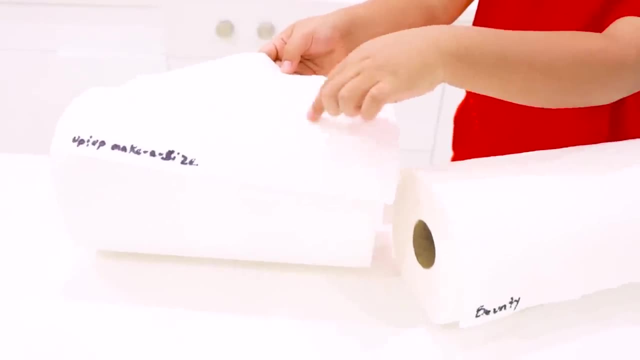 So now we took out the wrapper and we labeled them. So first we have the up-and-up and look, it looks a little bit different because like the lines and how it looks, And we got the one that I think is going to win too, the Bounty. 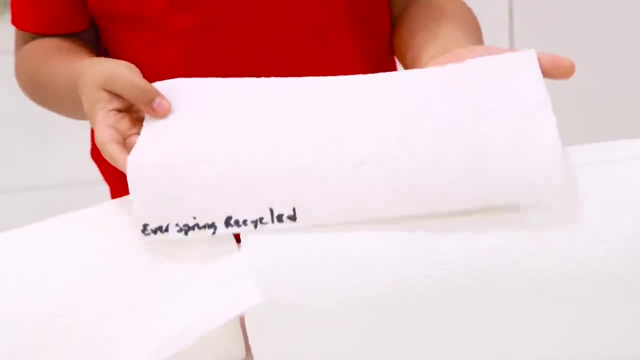 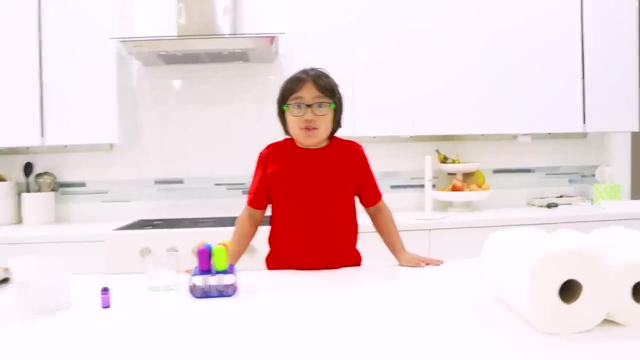 We have the Recycle one And look, it looks a little bit different than the others, darker, And we got the Bronte one. First I'm going to test which paper towel is more absorbent, So first I'm going to use purple. 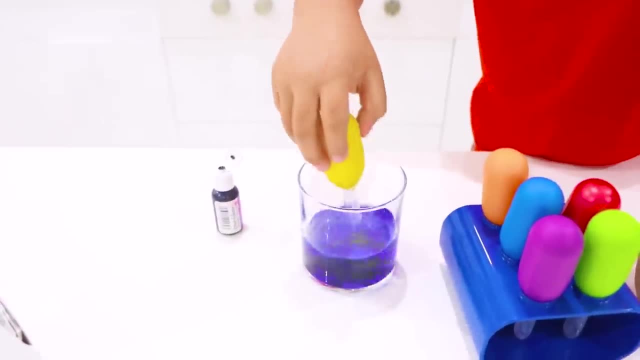 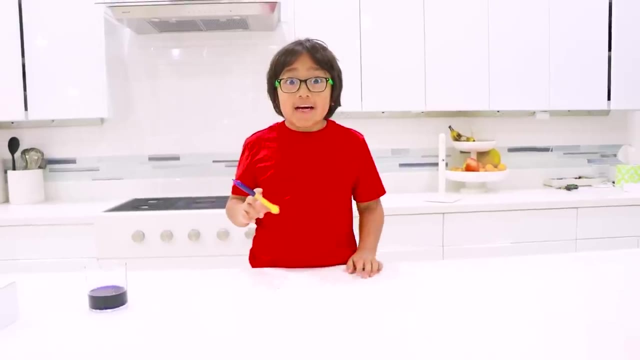 We can see better. Yeah, Okay, Perfect, Agitate, Agitate. So I'm going to put the same amount of water on the table. and don't forget to ask a grown-up for help. Ryan has a grown-up, Hi. 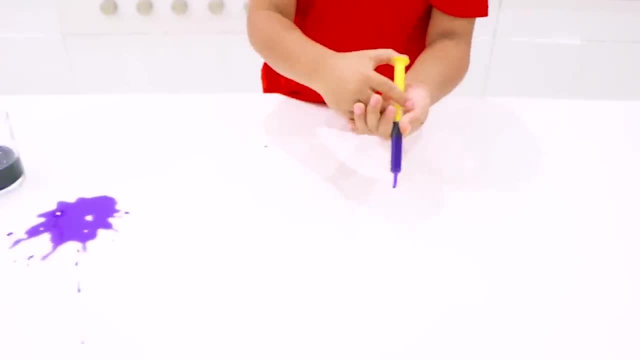 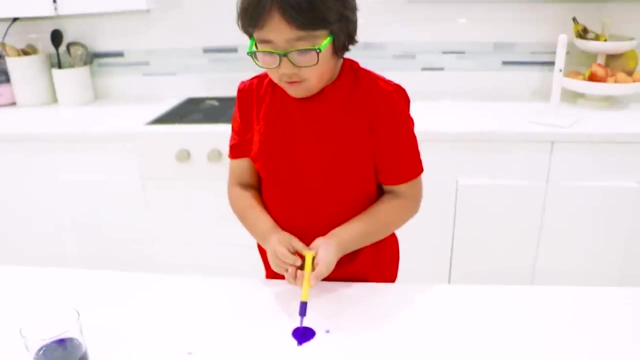 We're going to do four different spots to test out four different paper towel brands. Mm-hmm, Three, Four, Oh, Whoa. Now I'm going to put each brand of paper towel on top of the other one. Okay. 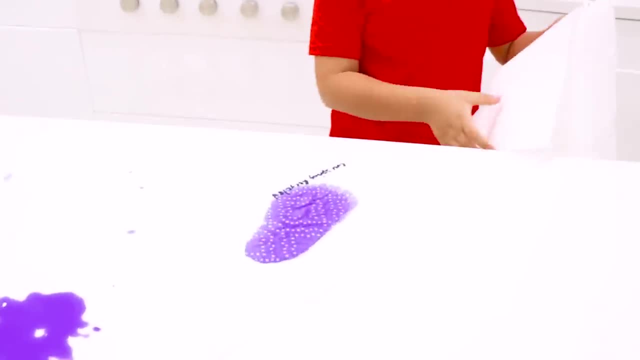 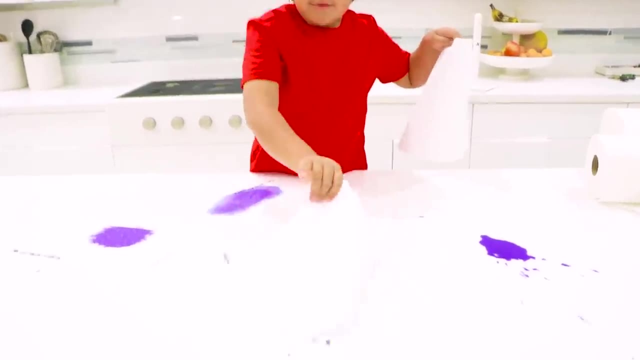 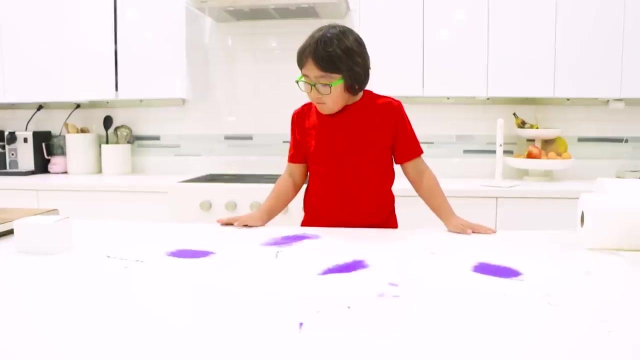 So we're just going to put the towel on each spot. This is the Recycling, this is the Up and Up. this is Bounty and this is Bronte. We're going to wait 60 seconds and we're going to see which one absorbs the best. 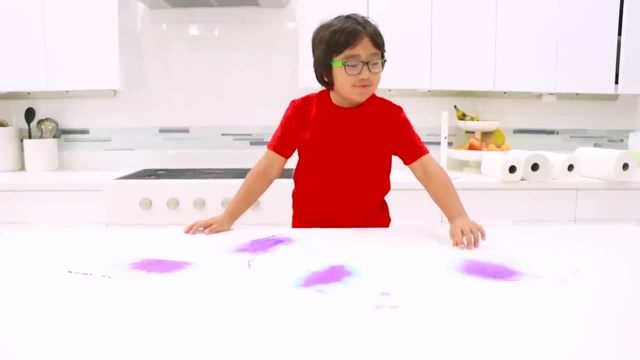 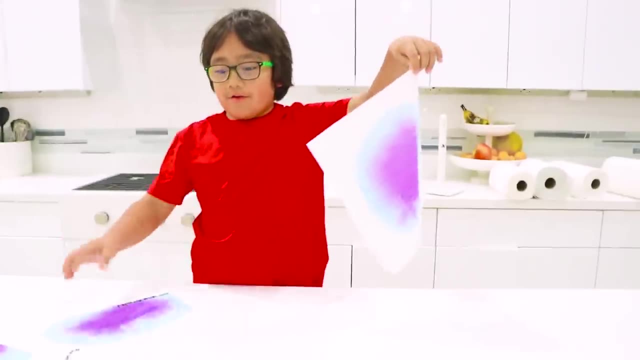 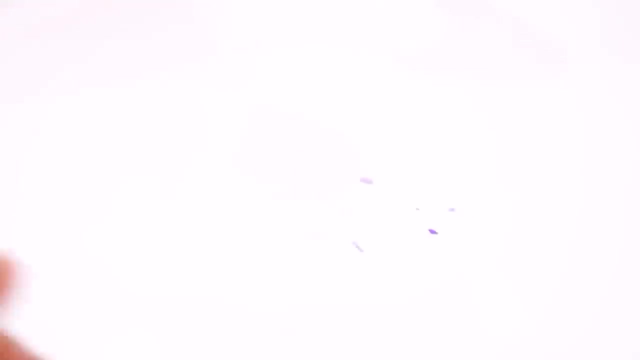 It's been 60 seconds, Let's see how they do. Whoa is the Bronte, so that one's pretty good. yeah, took away almost all of it. this one is the Bounty one. whoa, this one's pretty good too. oh, I think this one is better. this one, you can see a little bit. 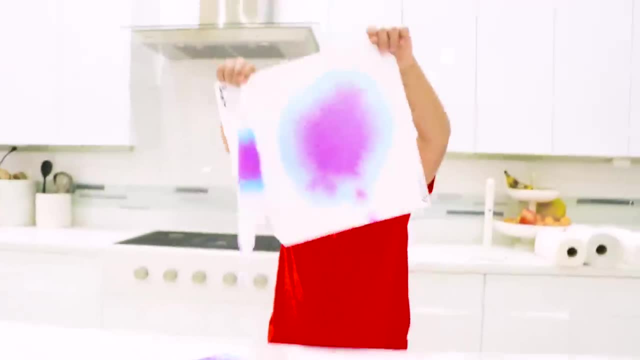 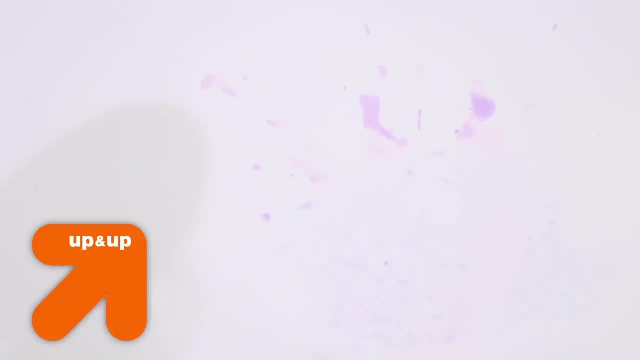 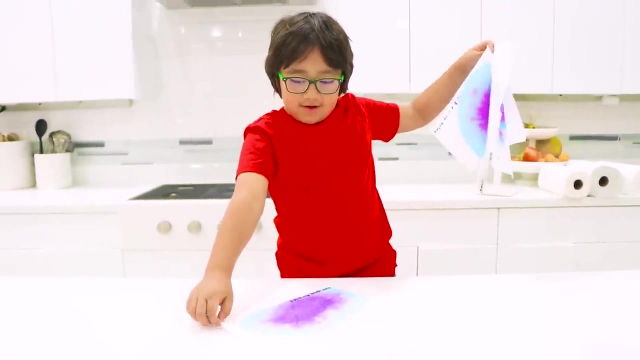 of wetness left, but this one is pretty much almost gone. so so far Bounty. that one is a Target brand. well, this one's pretty good too, oh yeah, but it still leave a little bit of wet spots here. so Bounty is winning, and this one is the Recycle one. oh, it's a little bit wet still, oh yeah, the. 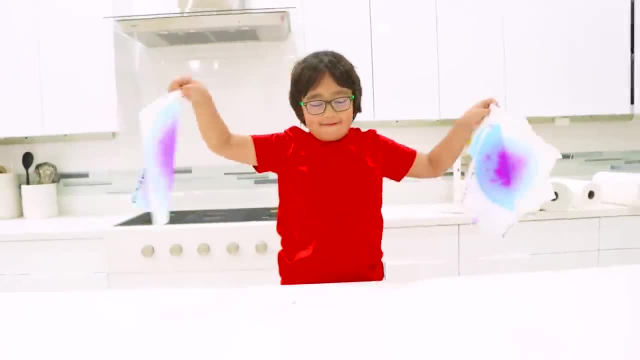 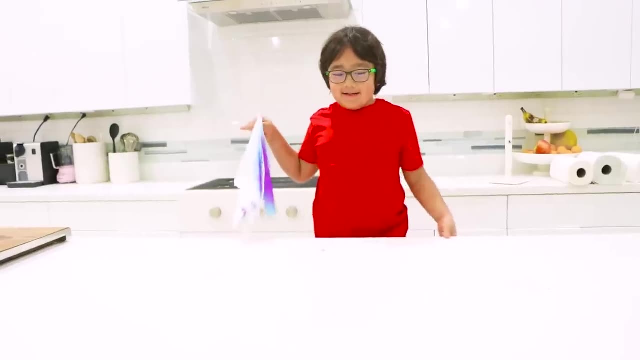 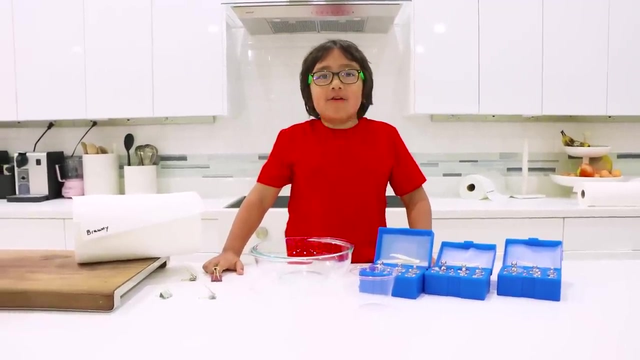 Recycle, one still left a lot of wetness. out of all the four brands of paper towel, which one did you think Ryan is the most absorbent Bounty? Bounty is the winner for round one is a big Bounty. next we're gonna test out which paper towel is the strongest. so first we're gonna 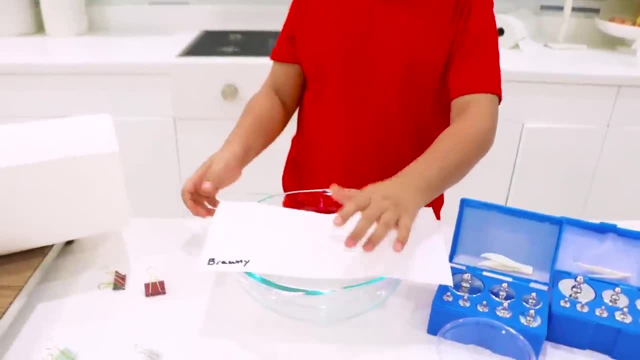 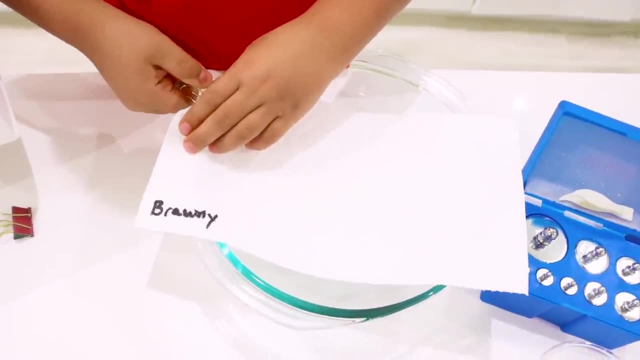 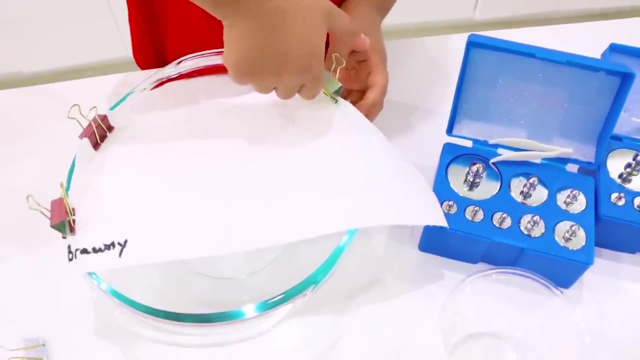 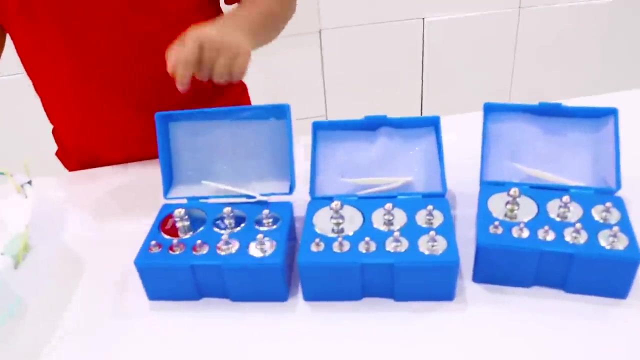 put Bronte on here, and then we're going to clip it on the other side. next we're gonna put on the cup and then we're gonna put on weights and we're gonna see how much weight it takes to break the towels. first, let's put 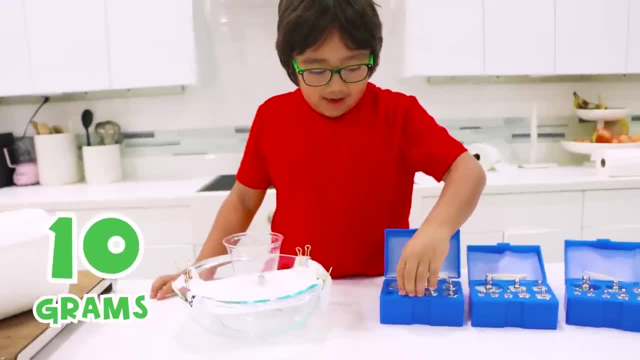 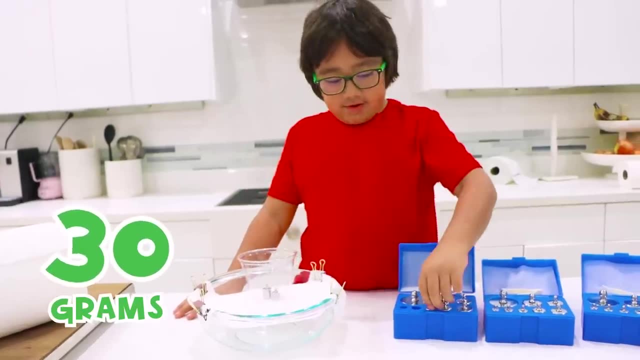 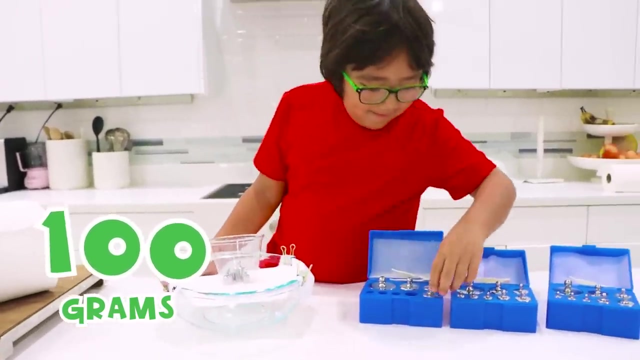 the 10 weight. Okay, nothing happened. Then what about we put the 20 weight, And then we're going to put another 21. And then 50. Ooh, so far, so good. And then 100.. Now we're going to put: 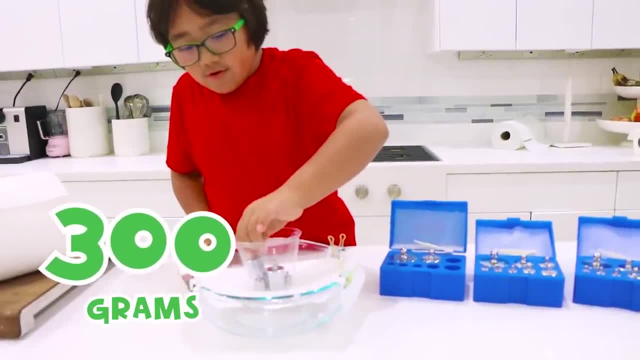 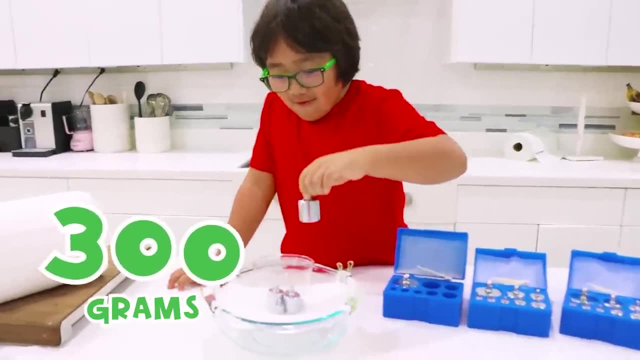 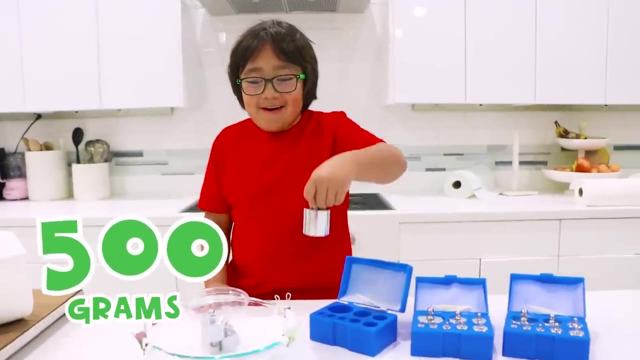 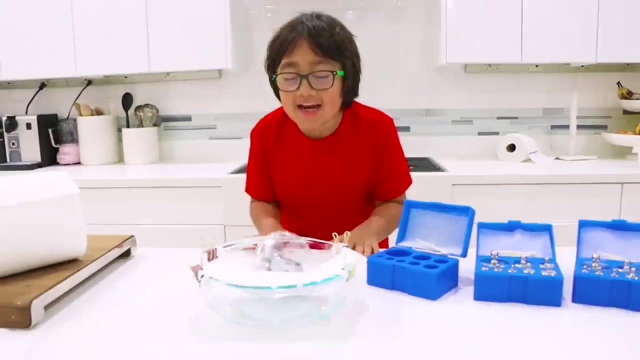 another 100.. Okay, Still good, And then the 200.. Ooh, We're going to have 500.. I think we have to put the 500 on. It's still still Dang. Look guys, the paper towel. 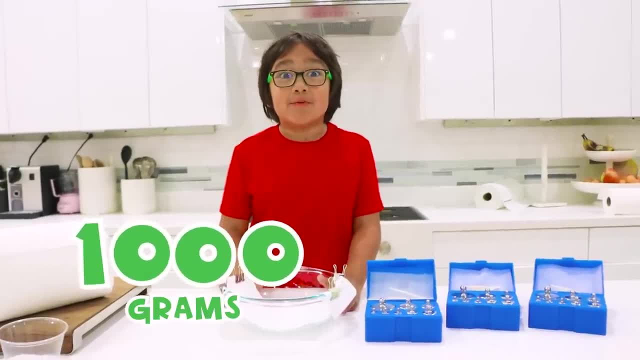 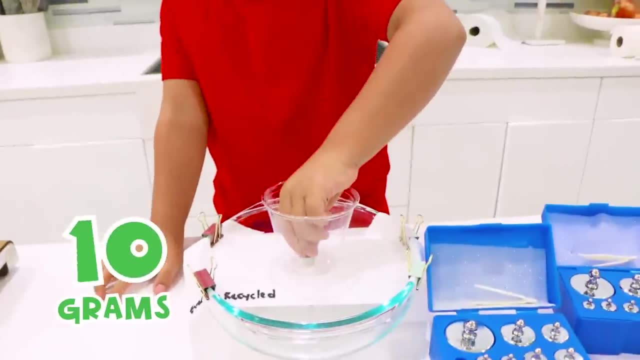 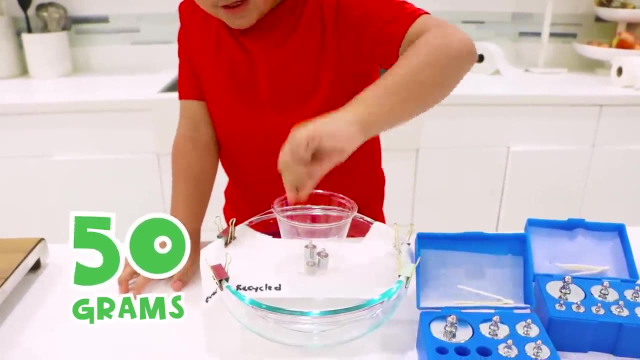 broke and it took 1,000 grams to break the paper towel. Now let's do the other one. This is the recycle one. So first we're going to put 10. And then 20. And another 20.. Okay, 50.. 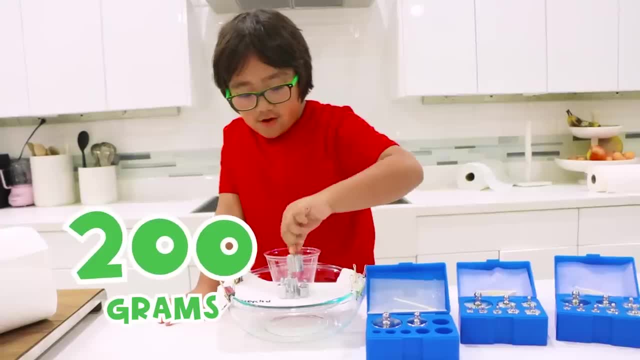 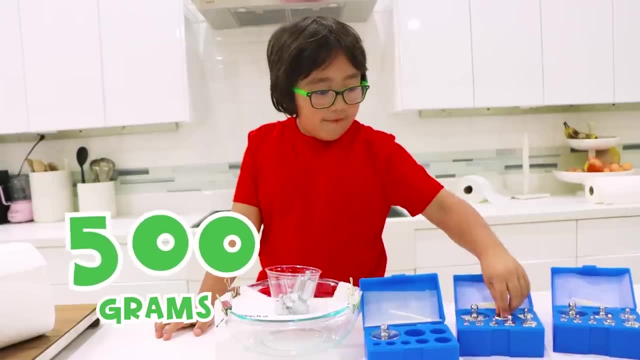 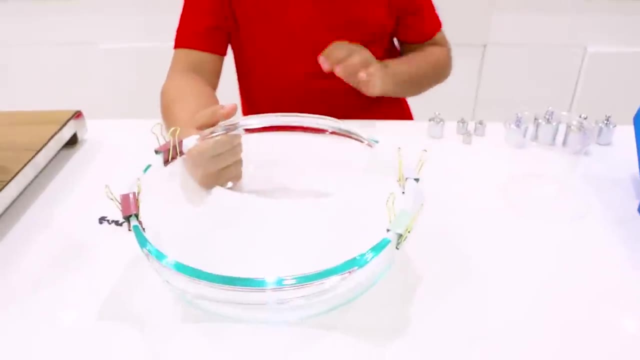 100.. Another 100.. 200.. Ooh, Let's put another 200.. Whoa, It broke The recycle one. It broke at 700 grams. Now let's do the next one. This one is the target up and up. 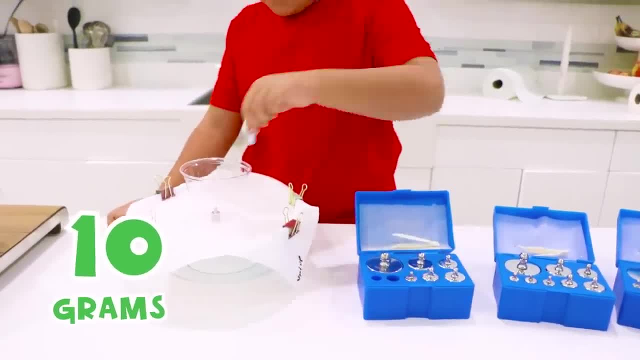 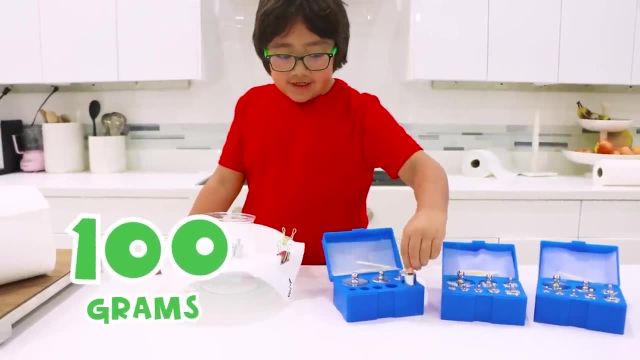 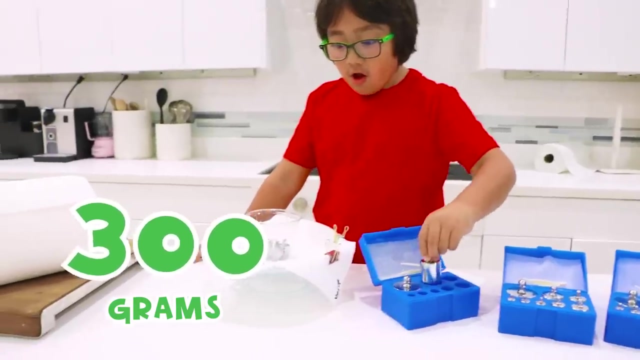 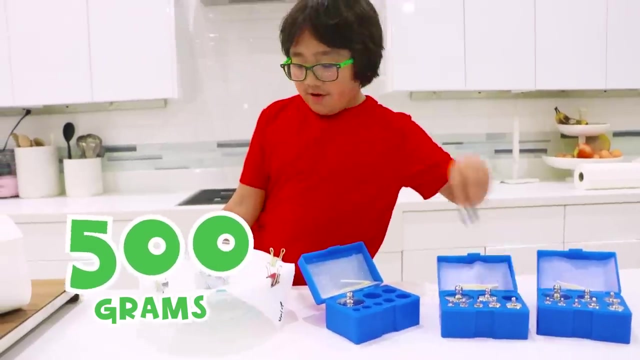 Now let's put the weight: 10. 20. Another 20. 50. 100. Another 100. 200. Okay, And then we're going to put another 100.. 200.. Okay, And then let's put another 100.. 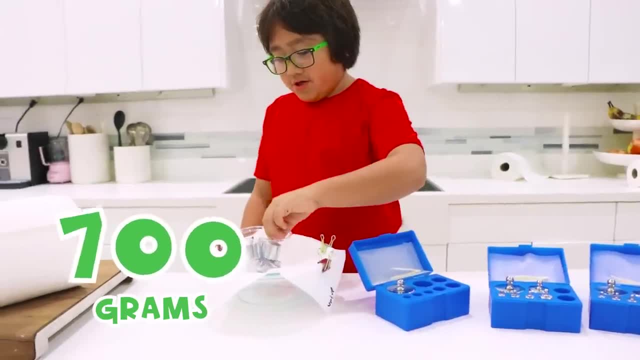 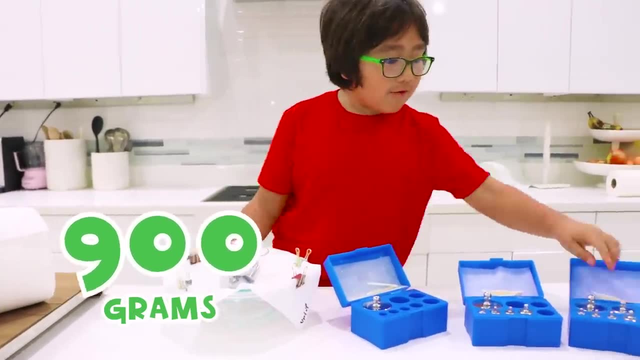 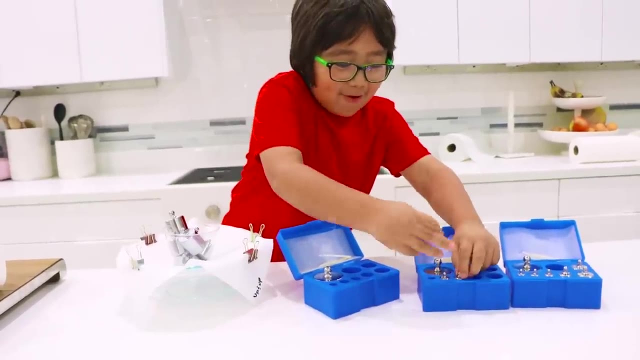 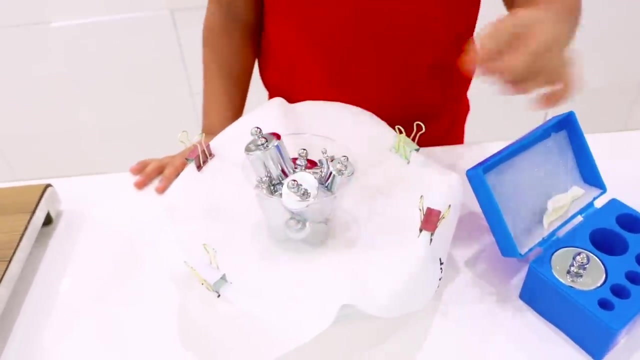 What about another 100?? Whoa, this one's strong. 200.. Whoa, 200. What? Okay, I'm just going to use all of these weights And see, when it breaks, What This is really strong. 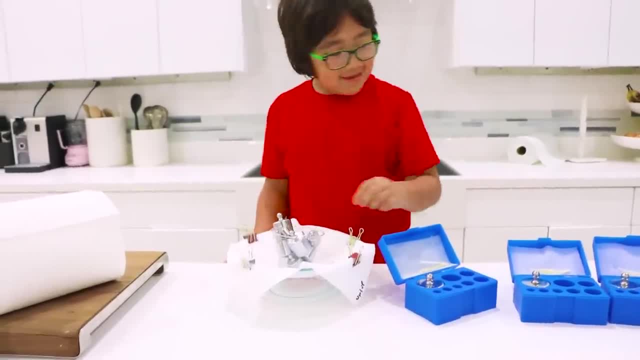 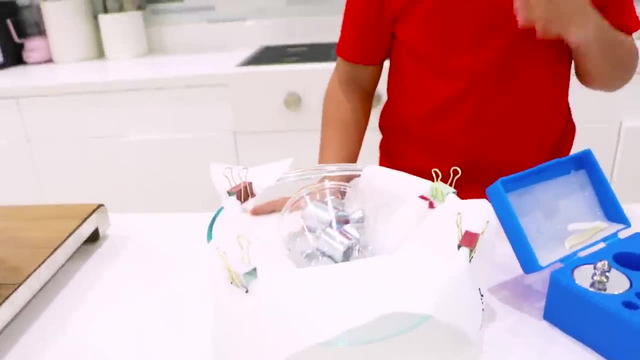 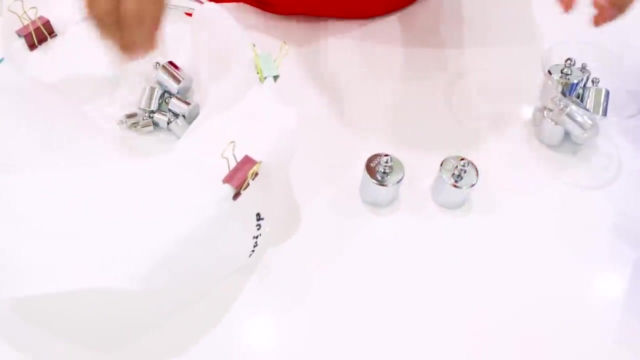 This is really strong. Wow, Target up and up. This is strong. Oh, it broke. Whoa. Okay, It could count all the weight. Look how much is left. This is a lot of weight. We're going to take them out and we're going to count them. 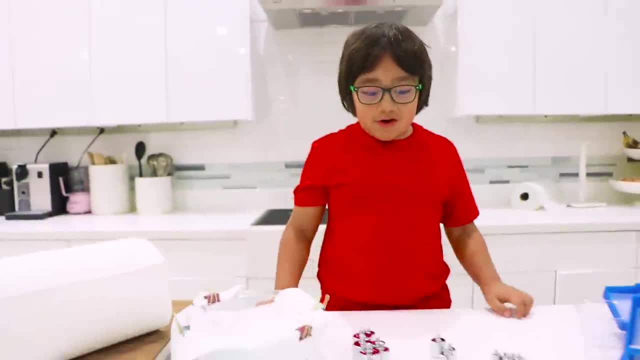 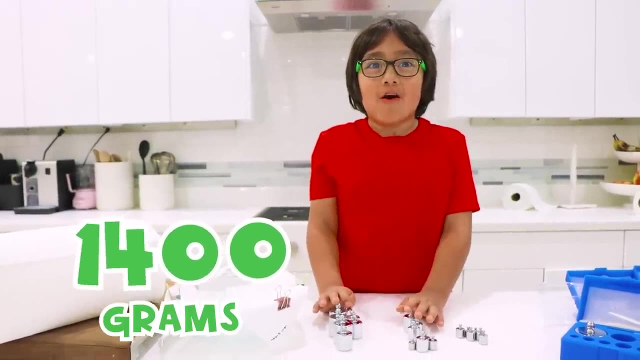 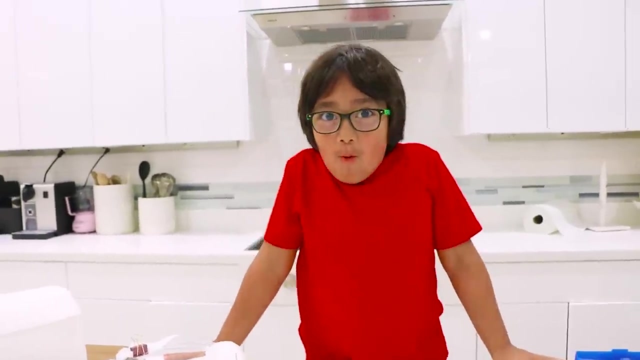 So this one broke, But it's the strongest because it has 1,400 grams. It's so strong. I didn't know Target up and up was so strong. Okay, guys, We're going to test out the last one. Let's see how it. 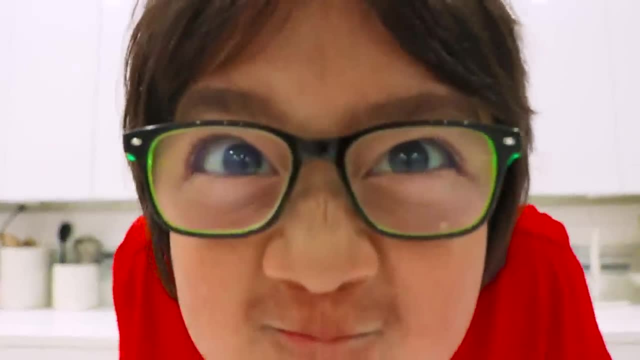 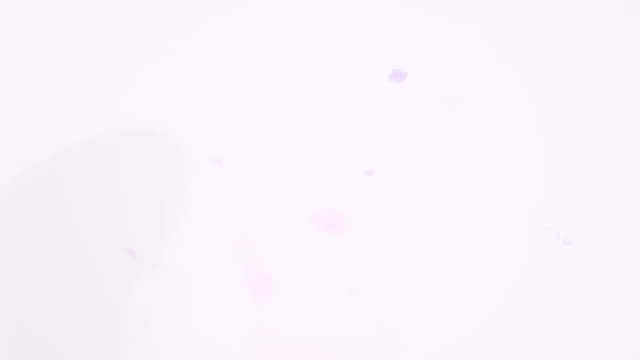 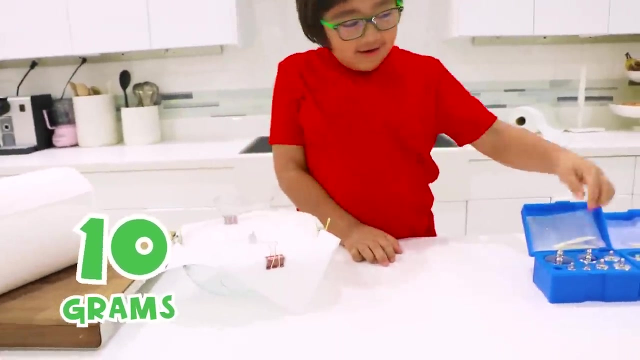 does Bounty. are you up for it? Last one, Bounty. Yeah, earlier we tested that the Bounty one was the most absorbent, But can it be the most strong? I think we'll find out, Okay, 10., 20.